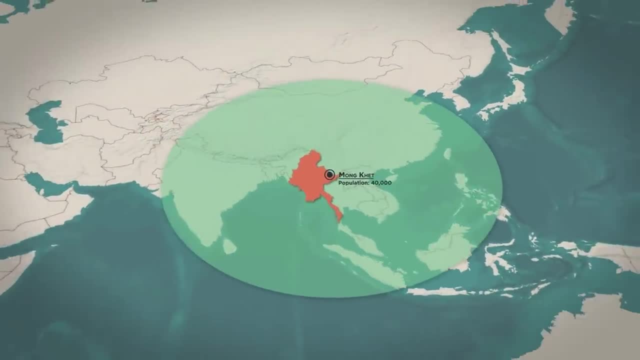 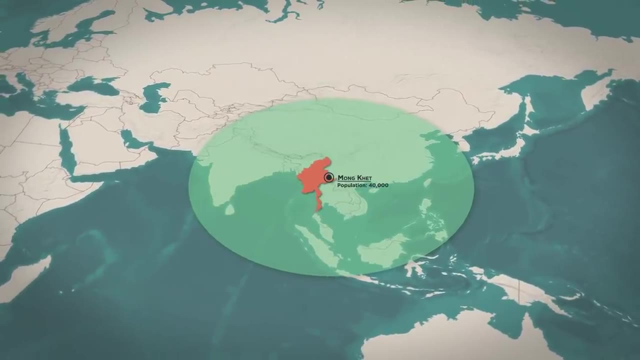 tourists. And yet if you drew out a circle from here with a radius of 3,300 kilometers, with Monquette precisely in the center, you will find that this is actually the smallest circle you could create that contains more people inside of it than outside of it. This fascinating 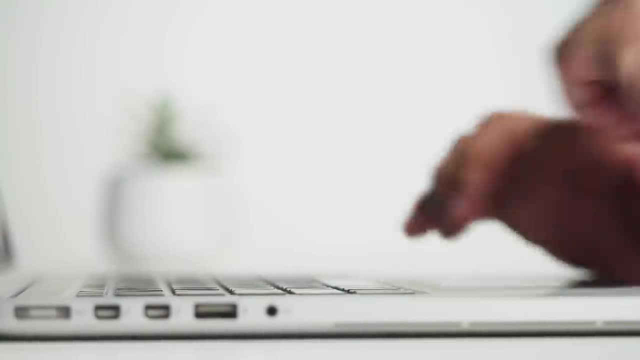 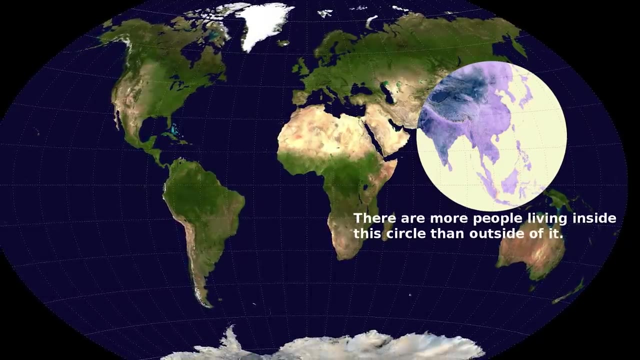 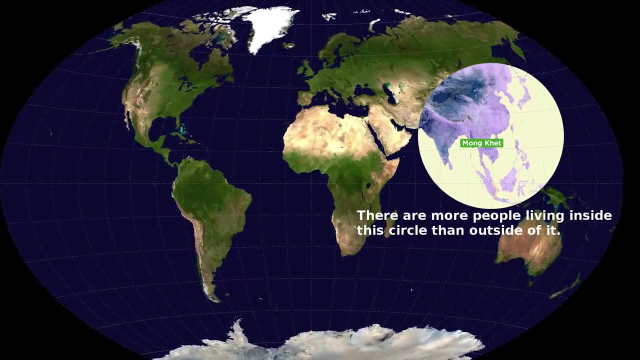 phenomenon was first realized back in 2013,, when a Reddit user going by the name of Valerie Pyrus and known in real life as Ken Meyer, posted a very similar map with a very similar idea that looked like this: Rather than Monquette, this map was centered instead over the South China Sea And with 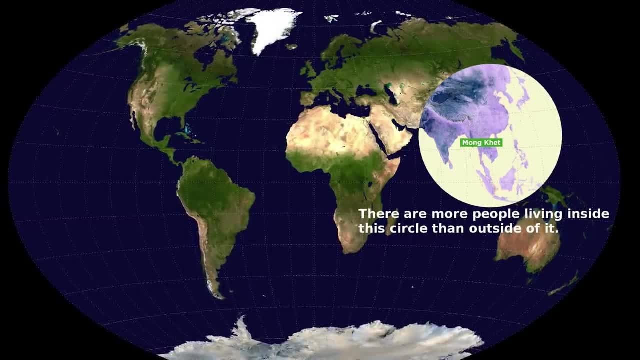 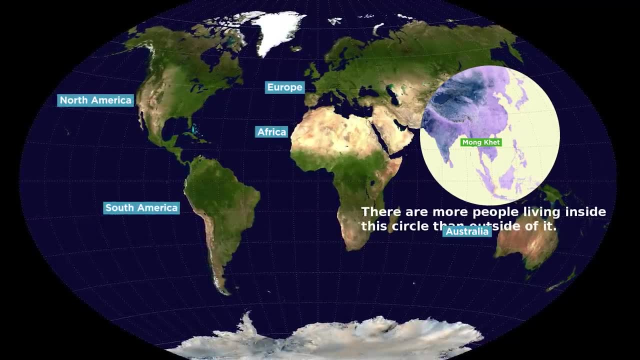 only a 4,000 kilometer radius. it only included parts of 21 countries and was shockingly small, Excluding the entirety of Europe, North America, South America, Africa, Australia and even most of Asia. entire massive countries like the United States, Brazil, Egypt and Russia were nearly. 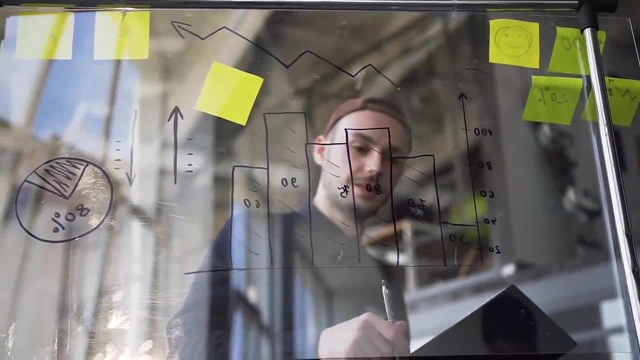 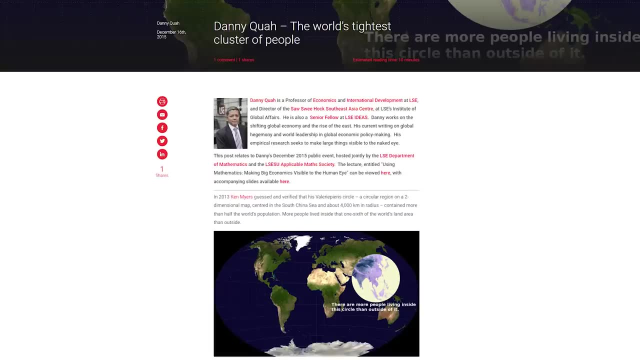 entirely left out And, as a result, the claim spread like wildfire throughout the internet and news media Ever since the claim has been backed up by nearly everyone, from the Washington Post to professors from the London School of Economics. So how does the math all break down? Well, for starters, the circle. 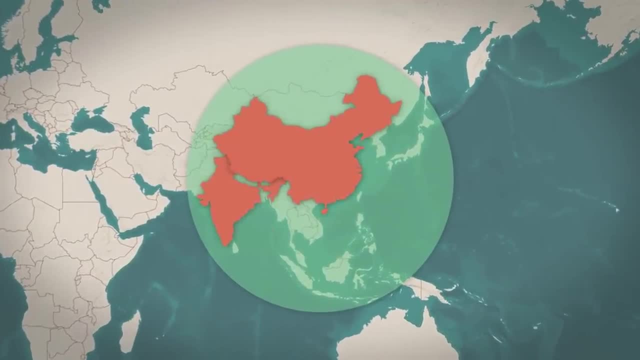 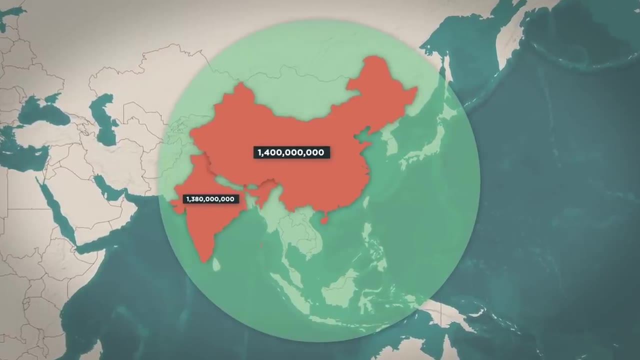 includes the entirety of China and India, the world's two most populous countries that, when combined, are home to 2.8 billion people and more than 35% of the entire human population. Already on their own, China and India are the only countries in the world that have a population of 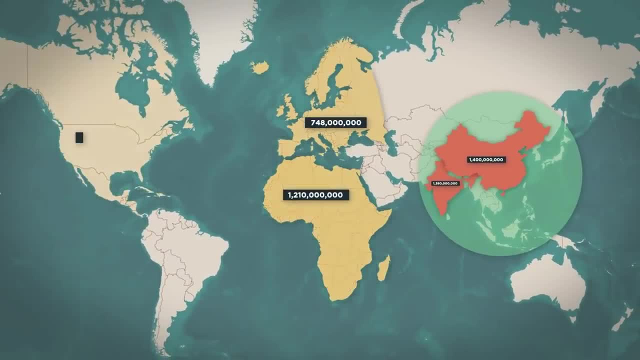 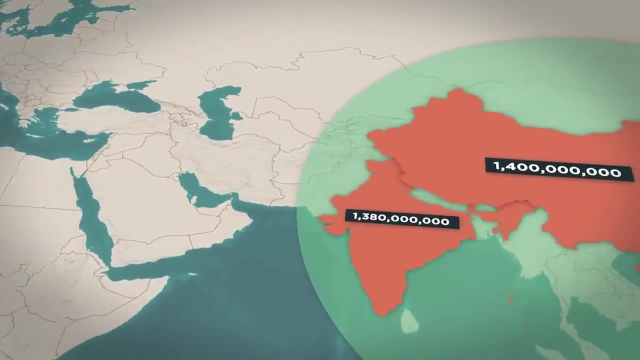 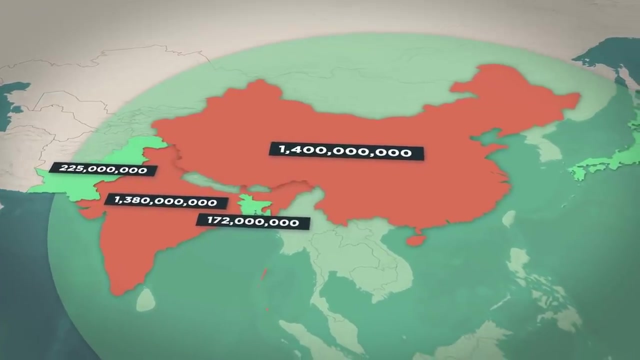 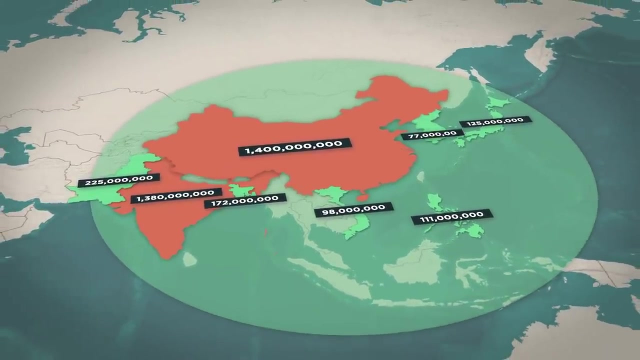 more than 1.8 billion people. So the total population of China and India combined have more people than the entirety of Africa, Europe, North America and Australia all combined. But there's many more highly populated areas within the circle than that. Most of Pakistan is included, with her 225 million people, Bangladesh adds 172 million, Japan adds another 125 million, The Philippines adds a further 111 million, Vietnam another 98 million, The Korean Peninsula another 77 million, While the Islands of Chaba, Sumatra and Borneo all add together another insane number of people. 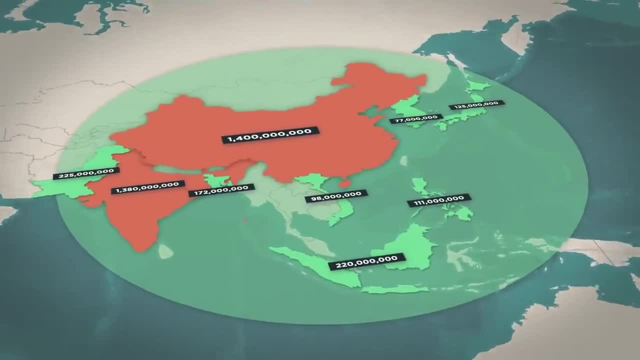 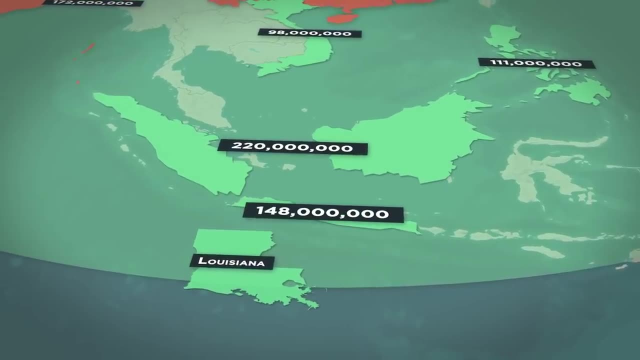 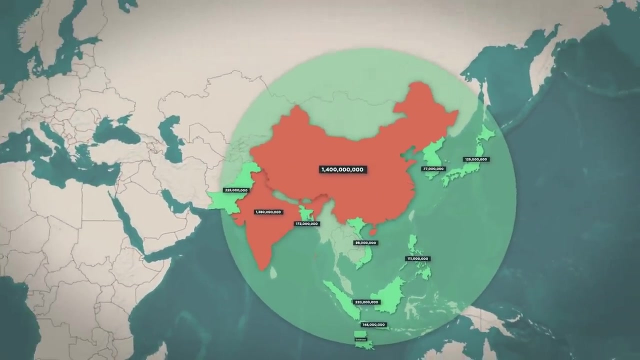 The small island of Java alone, roughly the same size as the US state of Louisiana, is the world's most populated island, with nearly 148 million people calling it home, which is a higher population than the entirety of Russia all crammed together on an island that's smaller than Louisiana. 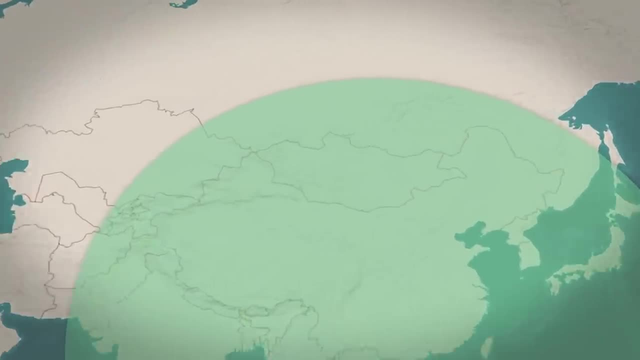 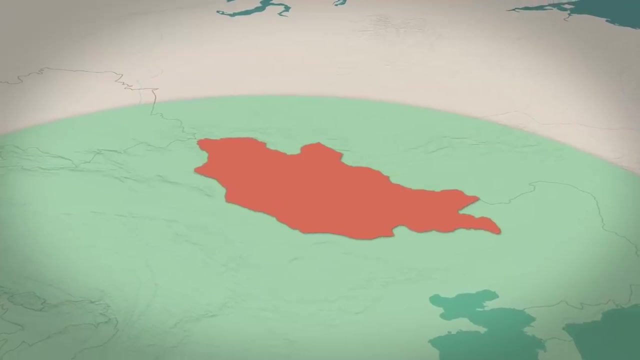 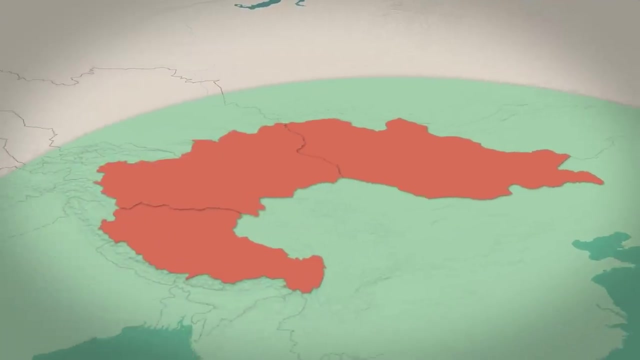 But what's also fascinating is that the circle also includes a lot of empty areas too. It includes nearly the entirety of Mongolia, the world's most sparse populated country, where, on average, you'll only find two people for every square kilometer of land. It also includes Tibet and Xinjiang within China, two areas that, when combined, 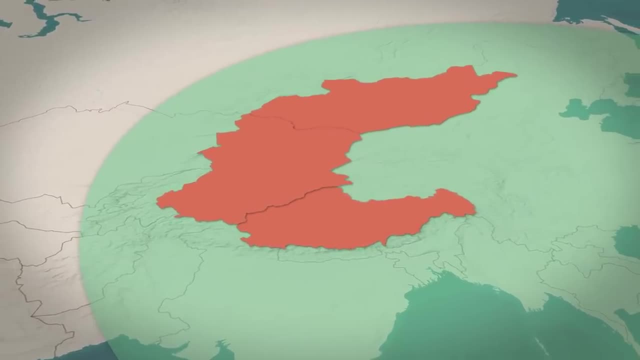 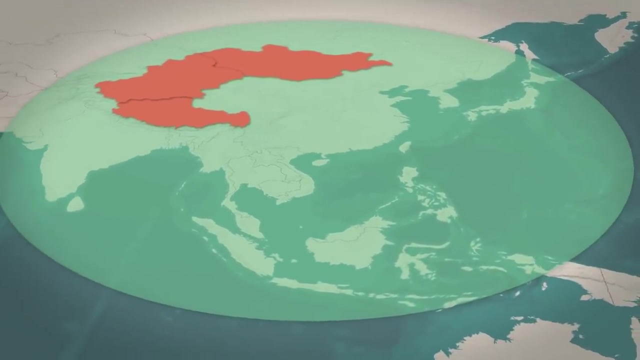 have a very similar land area to the entirety of India, but only being home to less than 30 million people. Further, the circle contains even more water than actual land, which, of course, is empty. And then, besides, just for the astonishing fact of its existence, the circle has many other. 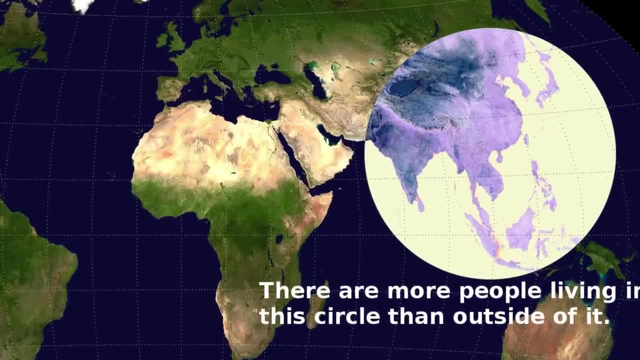 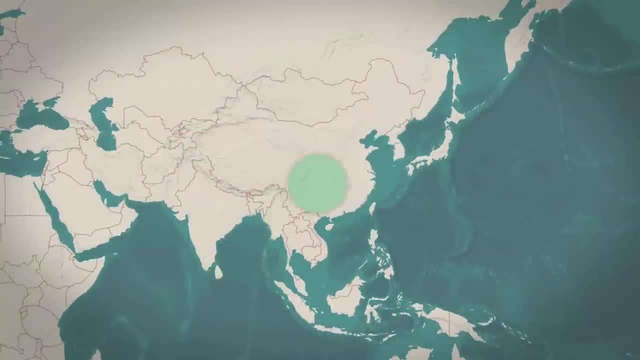 mind-blowing aspects to it as well. For one, there are many more Hindus, Buddhists and Muslims within the circle than there are outside of it. For Hindus and Buddhists that makes a lot of sense, but for Muslims it's pretty shocking, because the circle excludes the entirety of 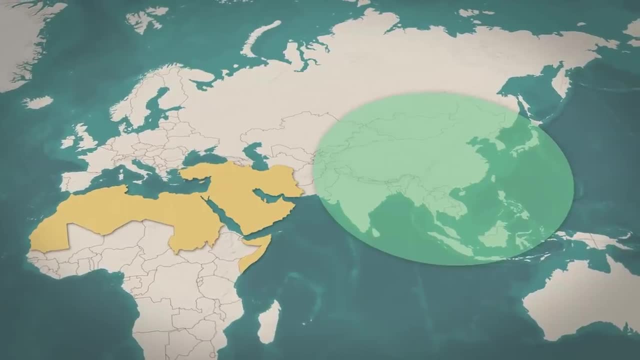 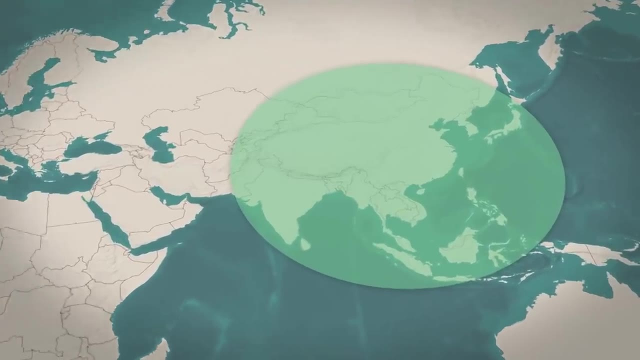 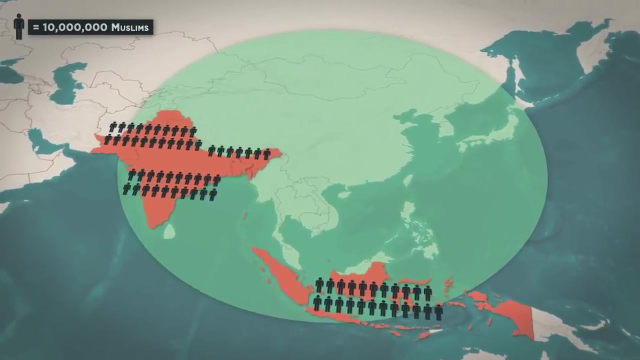 the Middle East and the Arab world, areas that are more often considered to be the epicenters of the Islamic faith. This is largely because of the enormous Muslim populations of just four countries that are largely within the circle: Indonesia, Pakistan, India and Bangladesh, which, when all combined, are home to nearly 800 billion Muslims. 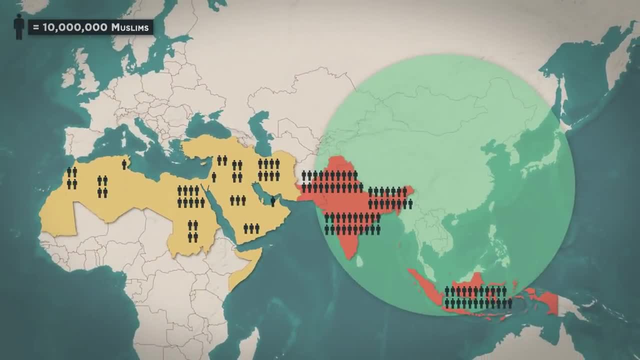 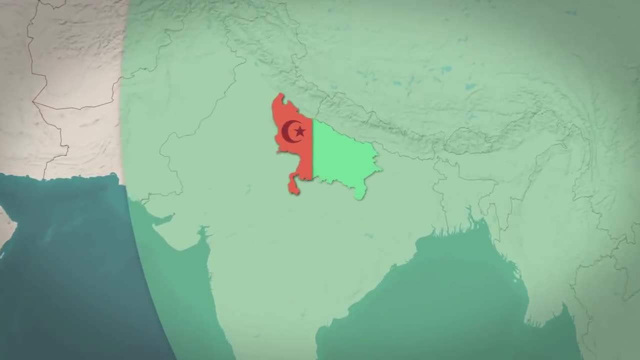 which is nearly twice the number of Muslims who live across the entire Middle East and North Africa. The Indian state of Uttar Pradesh alone has a Muslim population of only about 19%, But that's still nearly 44 million Muslims and is a higher Muslim population than any Muslim. 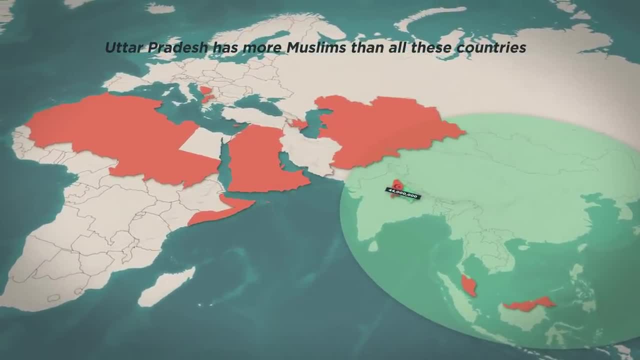 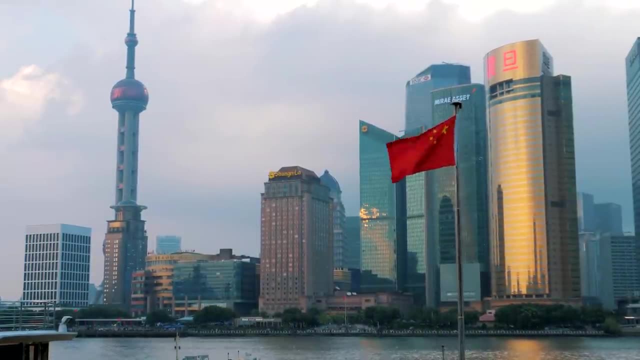 country in the world, besides for Indonesia, Pakistan, Bangladesh, Egypt, Iran and Turkey. Further, China has more Muslims than the entirety of Syria, and when you add them in, along with the tens of millions of other Muslims within the circle across Malaysia and the Philippines, you easily get to a 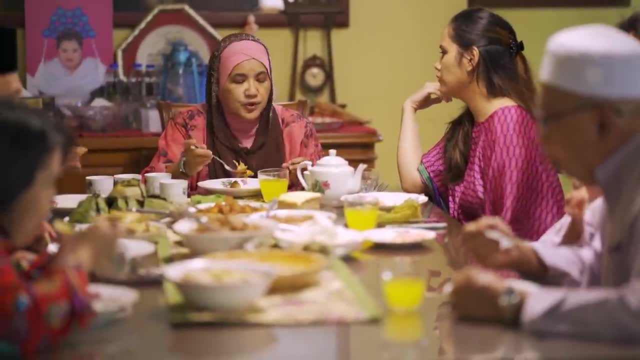 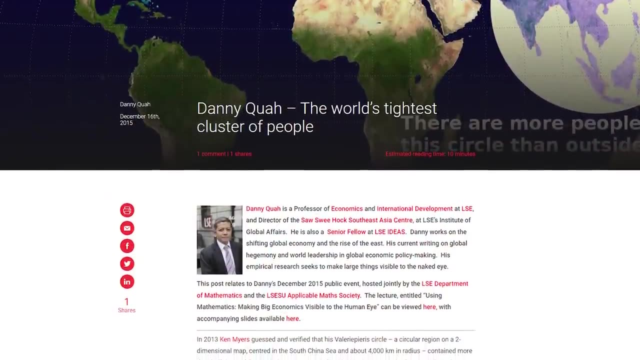 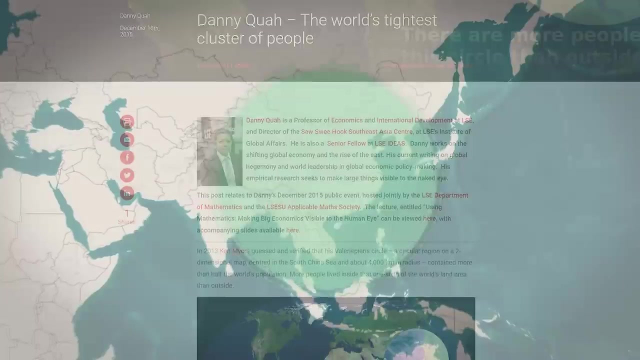 figure of more Muslims living within the circle than outside of it, making Southern and Southeast Asia the real epicenters of the Islamic population In 2015,. the Valerie Pyrus claim was verified by London School of Economics Professor of Economics and International Development, Danny Kwa but Kwa. 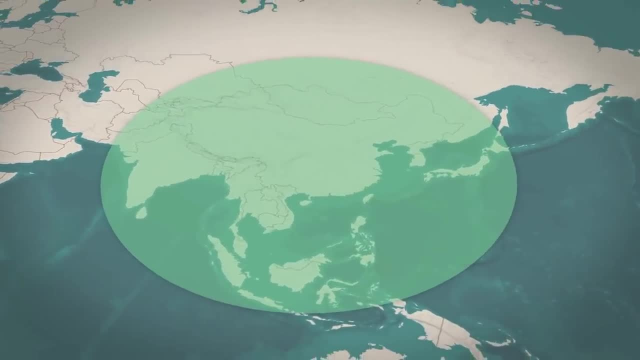 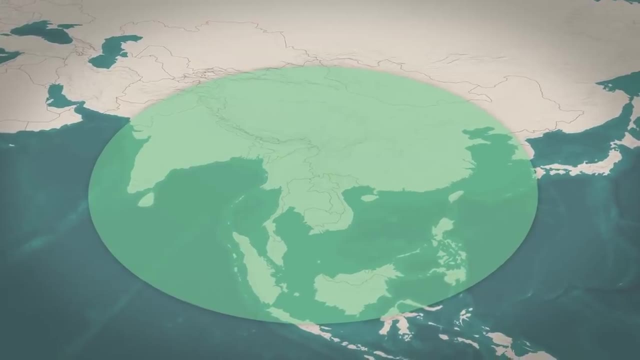 was interested in pushing the experiment even further, beyond Myers' original idea. He found that not only was Valerie Pyrus correct, but that if he adjusted the placement of the circle just a little bit, he could actually shrink it while having the inside of the circle still contain half of the 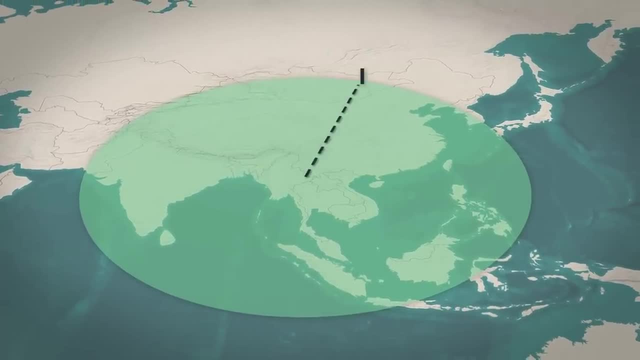 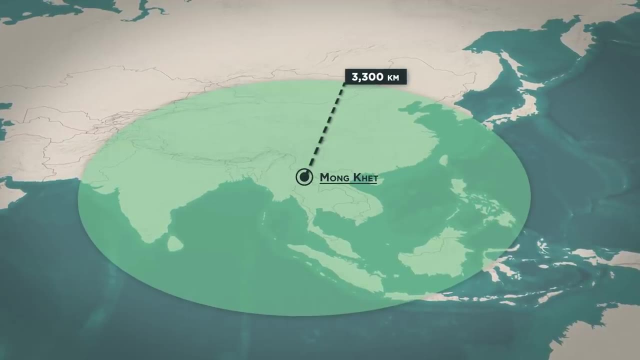 world's population. When doing this, he gave his new circle a smaller 3,300-kilometer radius surrounding the Burmese township Mongket, henceforth making Mongket the physical center of most of the world's population. Kwa's new map placed atop a 3D globe. 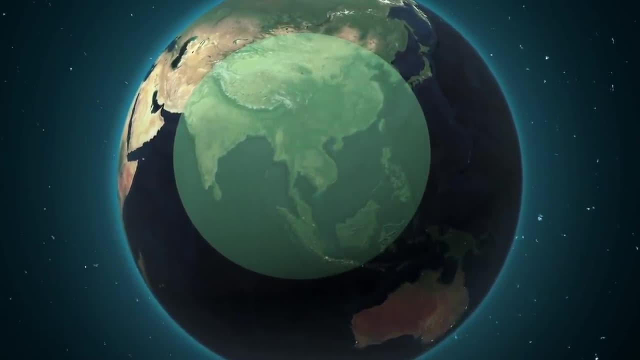 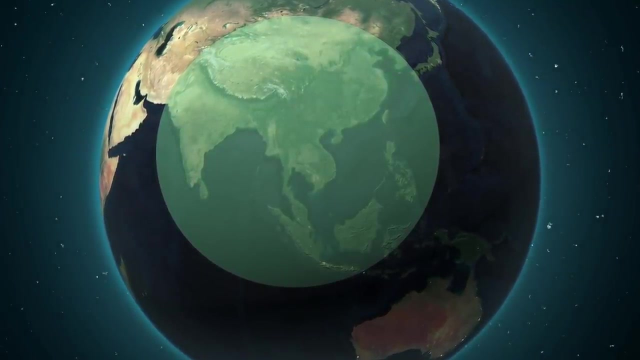 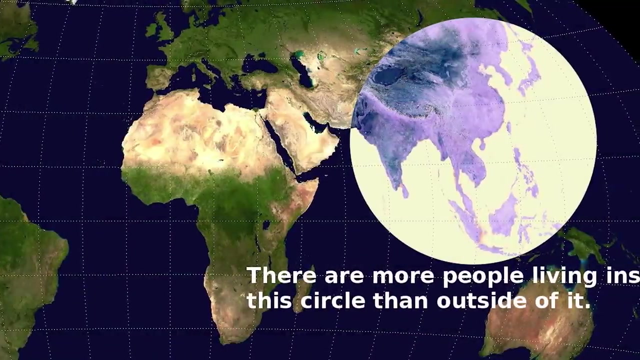 is even more fascinating. Half of the people in the entire world living right now are all inside of this small circle and, unlike the old map, it almost entirely excludes Japan as well, the world's 11th most populous nation. But the existence of the circle only begs another question. 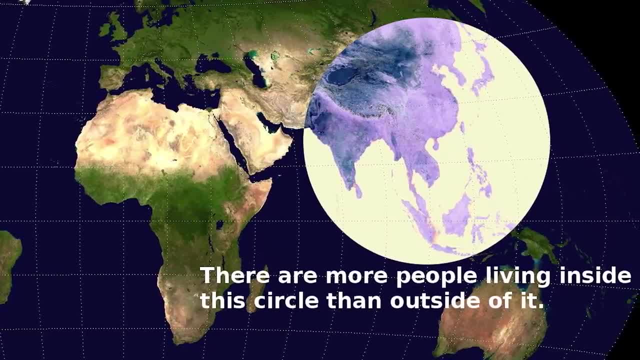 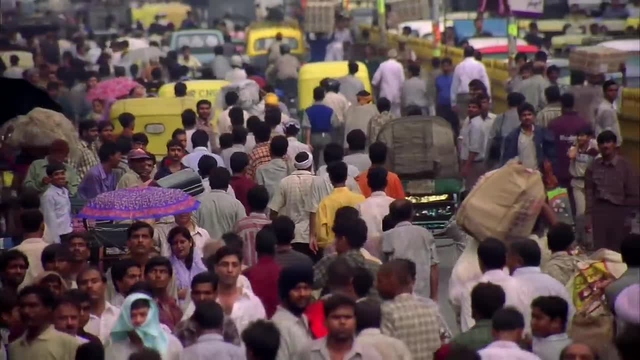 How did most of the world's population end up being inside of it? Well, the circle is centered over a large part of Asia, and this is where the majority of the human population is. So the total population has been now for thousands of years, at least as far back as 1000 BCE. The 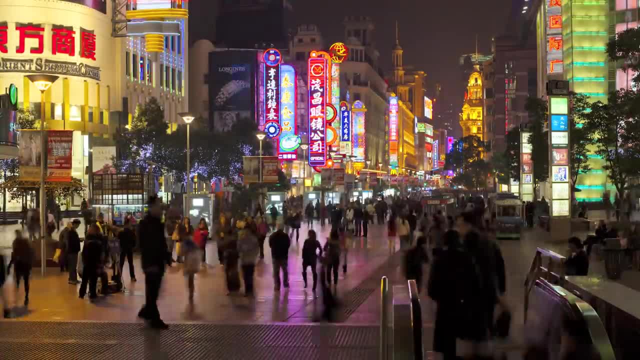 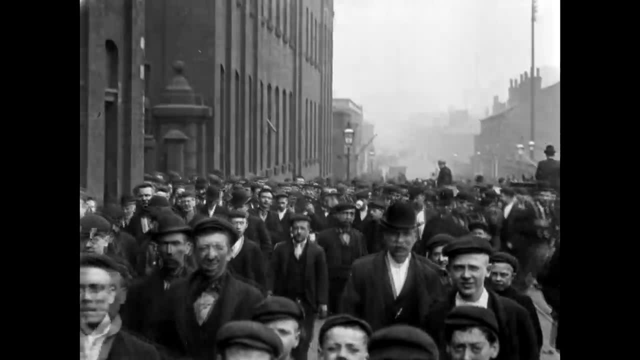 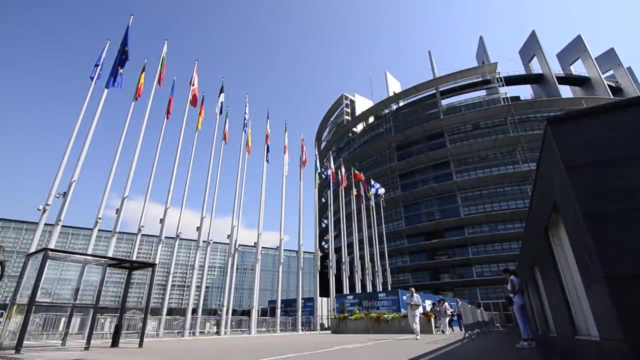 closest that any other continent has come so far in the past 3,000 years to Asia's population was Europe at the turn of the 20th century, and even then Europe's total population was only 43% of Asia's total population. Fast forward 120 years to the present and that percentage has shrunk. 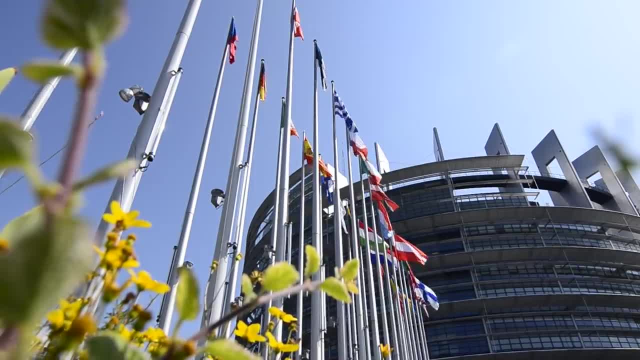 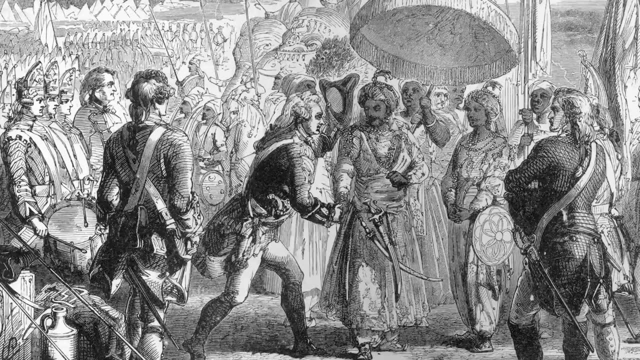 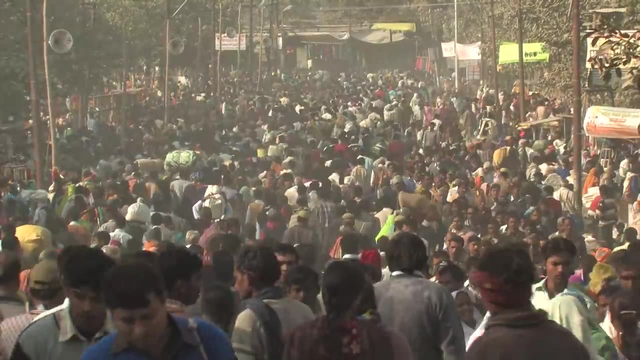 down to less than 17% of Asia's population today. Even if you go all the way back to the 1700s, India and China alone accounted for a little more than half of the entire world's population, with more than 150 million people each And over the three centuries of history. 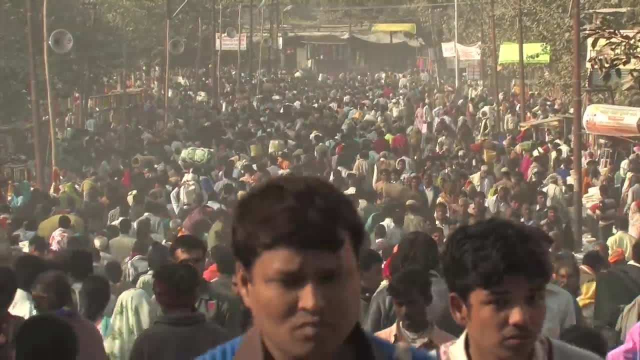 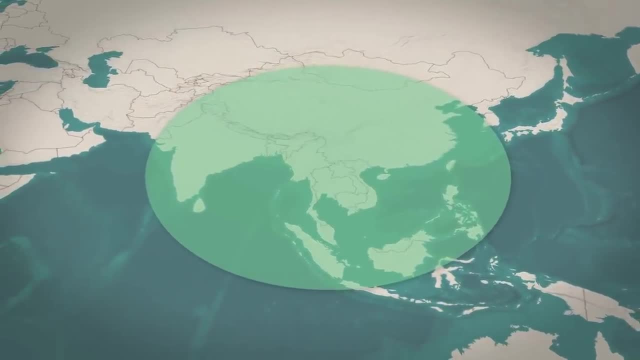 since both have added more than 1 billion additional people. So, for about the past 3,000 years, this small circle that contains the majority of humanity has remained more or less constant in the same general location, Despite both adding more than a billion people to their 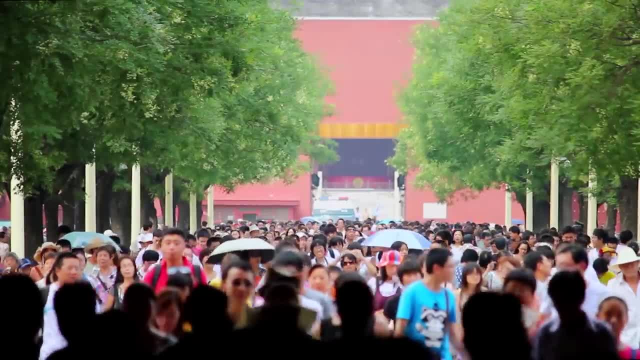 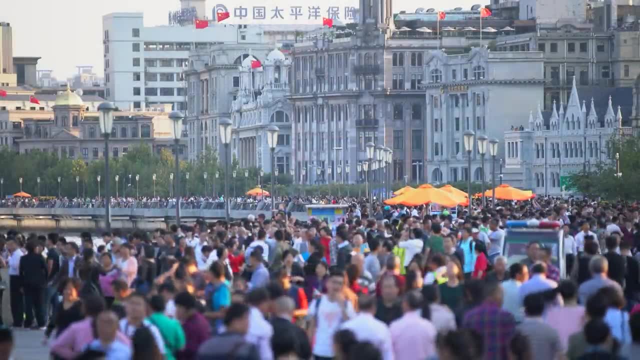 populations. India and China alone have accounted for a little more than half of the entire world's population. However, both India and China have been growing at more or less the exact same rate as the rest of the world over the past 300 years. That trend ultimately means that both India and China have so many more people than any other country today because they had so many more people than any other country did 300 years ago as well. In short, they simply had a much larger head start than any other country did. But like, okay, that doesn't really answer anything. The 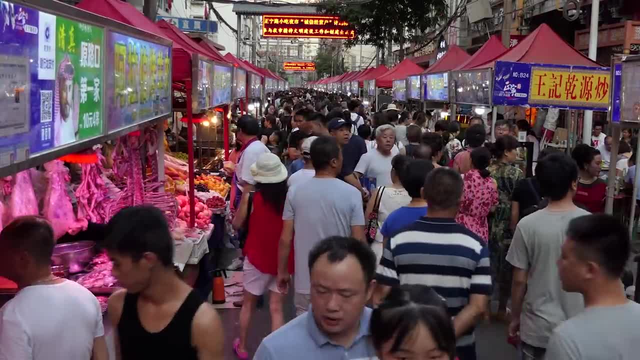 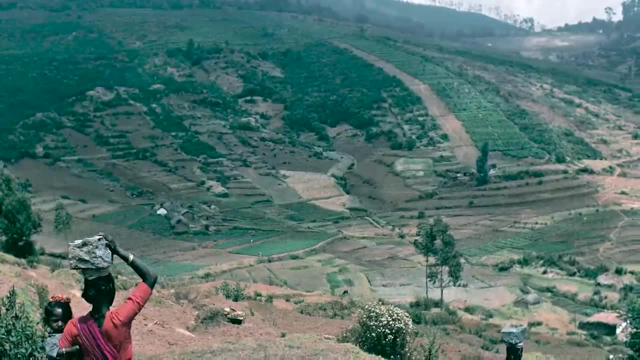 real question is: why did they have so many more people than any other country did 300 years ago? The real question is: why did they have so many more people than any other country did 300 years ago? The big two answers to that question are land and food. China and India measured by land. 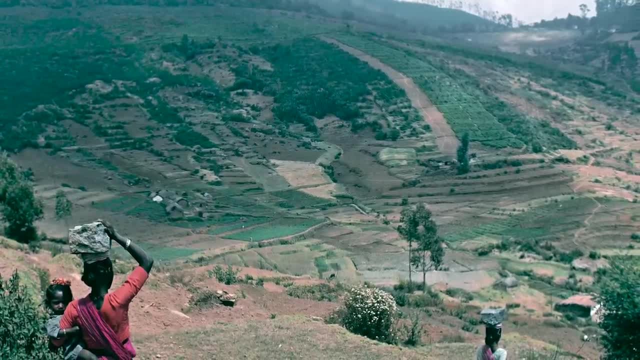 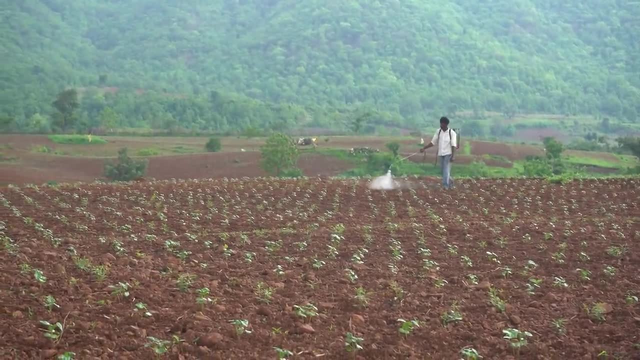 are both massive places and they both have large rivers that flow across easy-to-farm plains. Modern India has more arable land than any other country in the world And, unsurprisingly, China has the fourth highest amount, behind Russia and the United States. 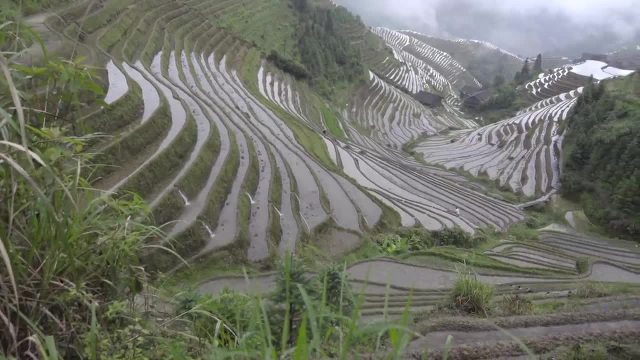 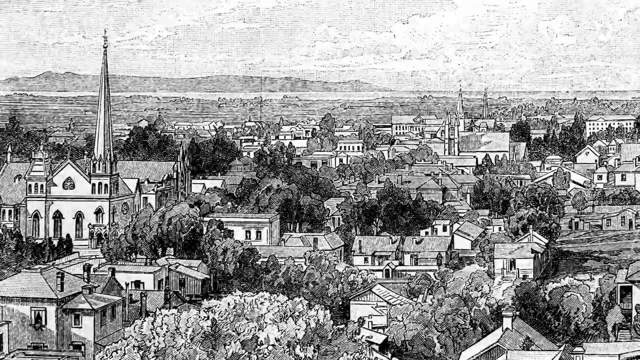 The reason why China had more people than either of those countries 300 years ago, though, is that Russia has a bit of a problem with the cold, and they mostly can't grow crops year-round, while the United States just simply didn't exist yet, So, once again, China simply had a bigger head. 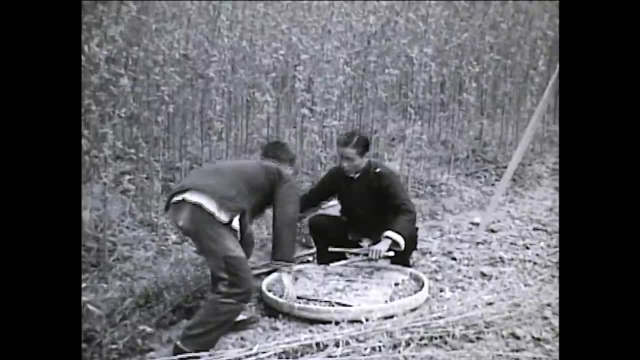 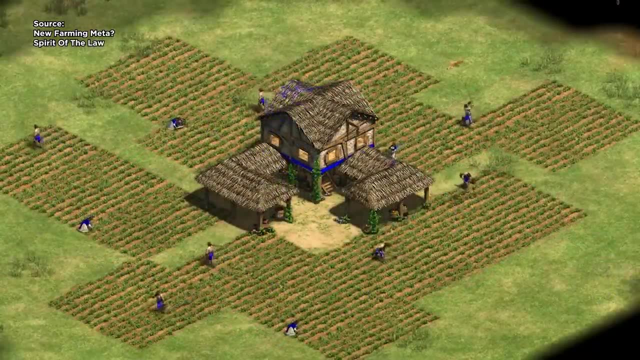 start with thousands of years of farming and development over both Russia and the United States. All of this arable land, combined with the ability to grow crops on it year-round, enabled both Indian and Chinese civilization to simply be able to plant more farms than anywhere else, which meant 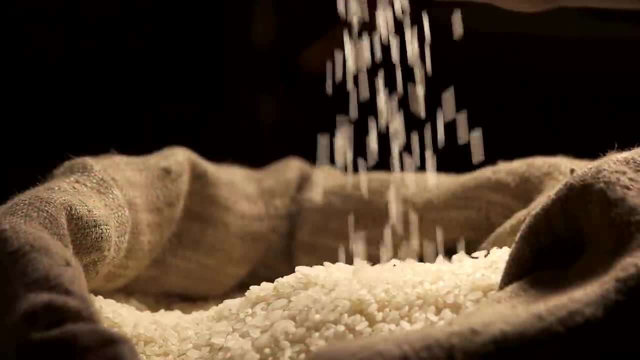 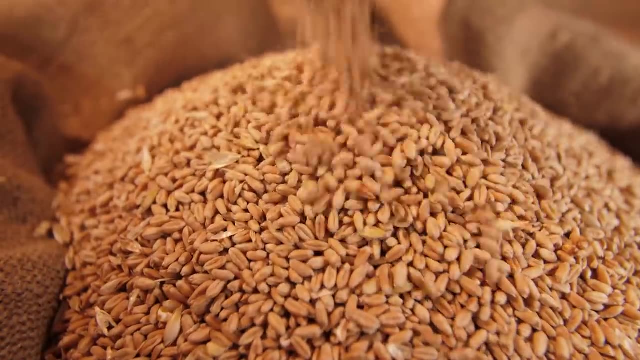 more villages and so on, And the crop that these places were primarily growing was rice, which, when compared to other popular grains like wheat, contains significantly more calories per acre For most of human history, and then even into the present, the most popular grain that was grown. 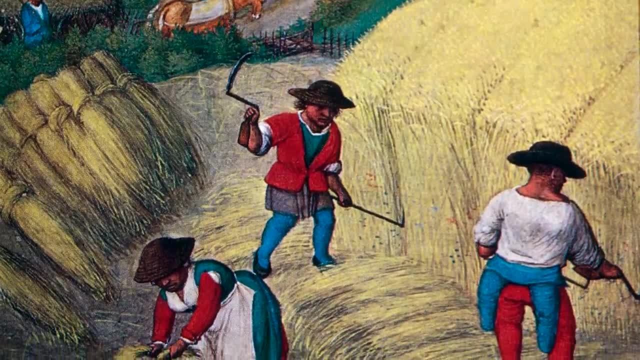 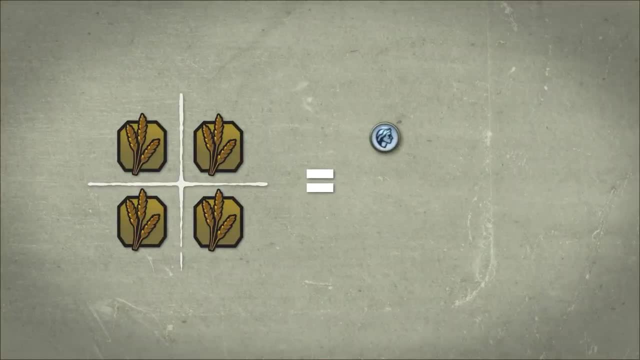 across the Middle East and Europe was wheat, which only produces about 4 million calories per acre. That means that for every acre of farmland growing wheat, a civilization could only feed a little more than six citizens a year. Now, if you want to know more about this, be sure to subscribe to our channel and hit the bell. 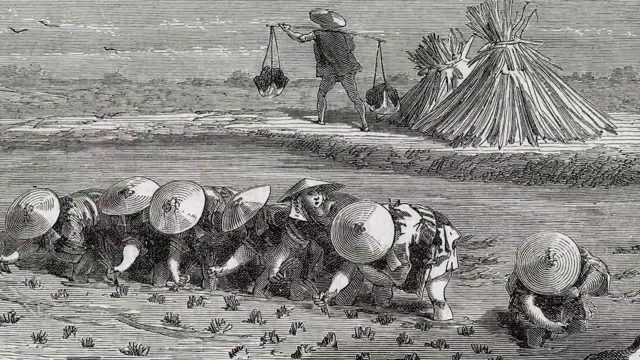 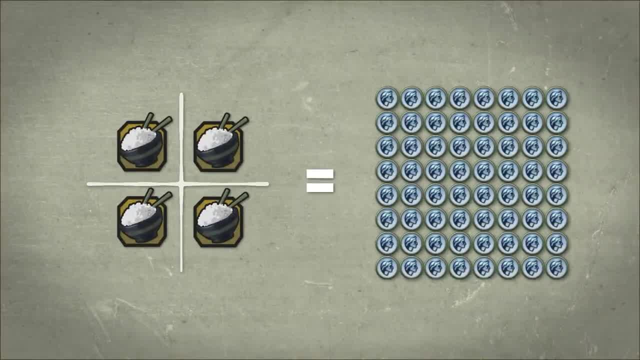 so you don't miss any of our new videos. And don't forget to hit the bell so you don't miss any of our new videos. Conversely, rice generates more like 11 million calories per acre, which means that when a civilization uses rice, every acre they use can feed more like 16 people. 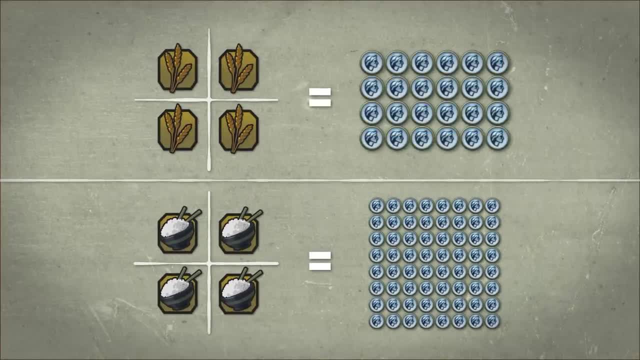 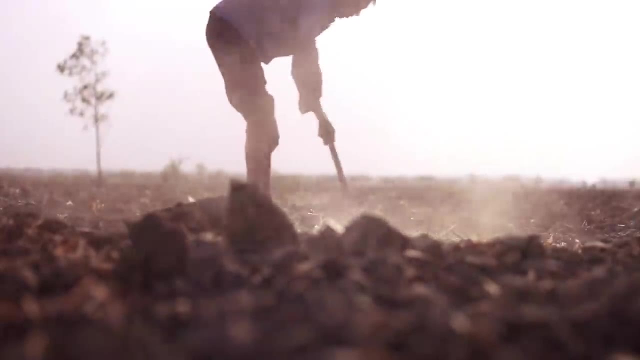 The choice between wheat and rice is obvious for population growth. When civilizations choose rice, as China and India and the other countries of East and Southeast Asia have, their acres of farmland can simply sustain more people than the civilizations who choose to farm wheat, And when they have the first and fourth highest amount of 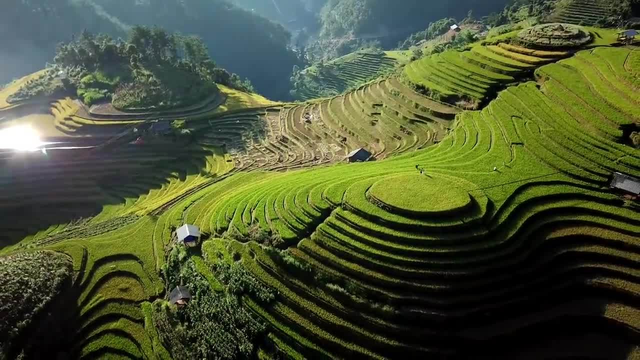 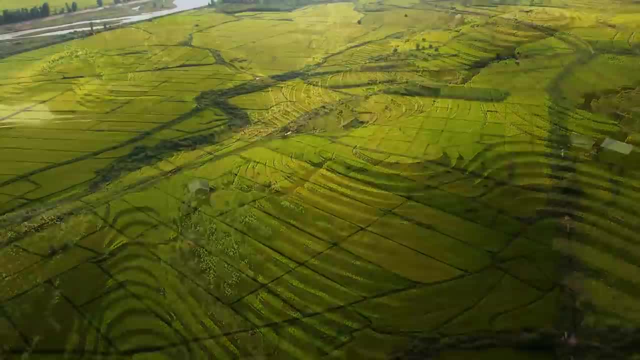 available farmland in the world and they have the climate to farm year round. it's not exactly hard to figure out why they've literally always had the highest number of people and will continue having the highest number of people for a very, very long time. 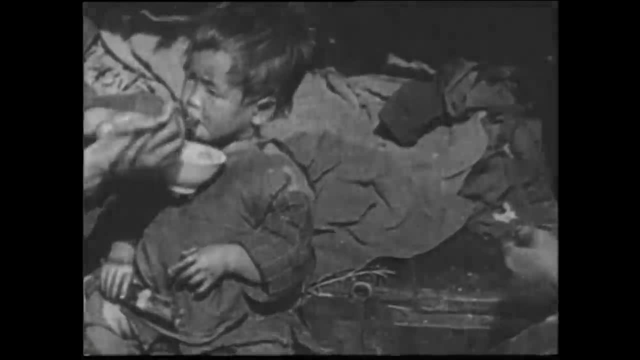 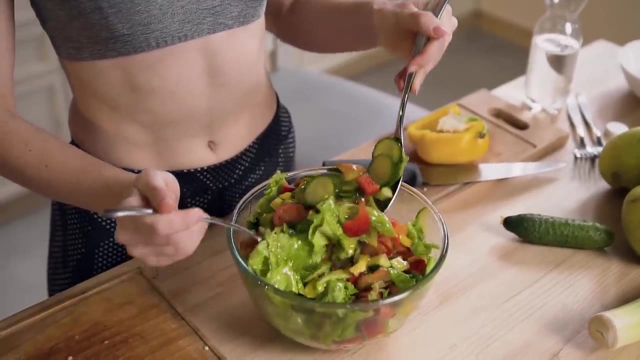 A higher source of calories in the form of rice over thousands of years is one of the major reasons for the higher population of Asia today And, on a personal level, having easy access to good, healthy food is one of the primary factors to living a good 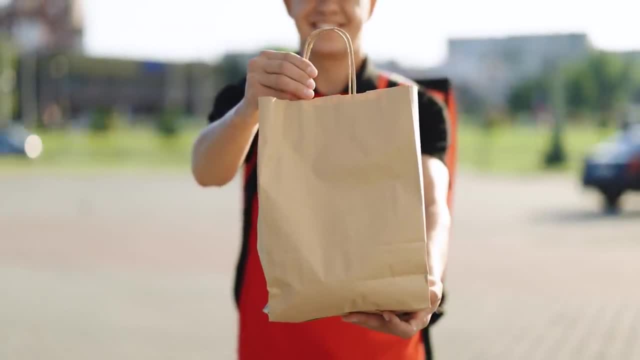 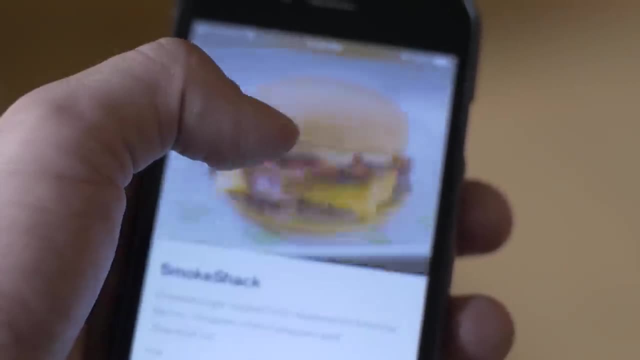 healthy life. Ordering great tasting food via delivery or takeout is definitely easy, but with all those fees added on by the apps it becomes pretty expensive to have food delivered straight to your door. But many of us still do, because it's simply convenient. I definitely did. 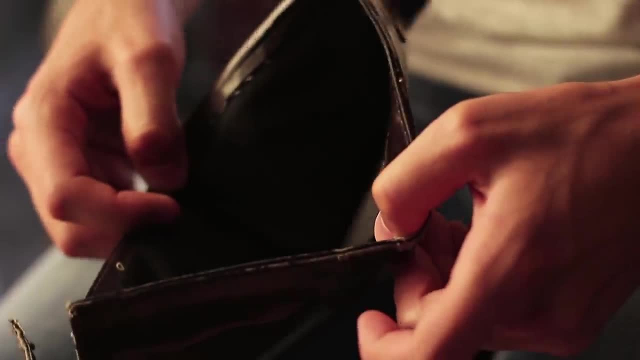 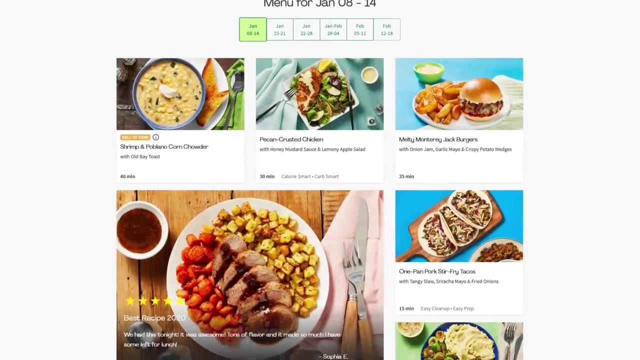 until I realized how poor it was for my health, for my wallet and for the environment. Therefore, I eventually switched to using HelloFresh. Now I just go to HelloFresh's website, choose from a list of 50 weekly menu items, pick what I want and then the following week 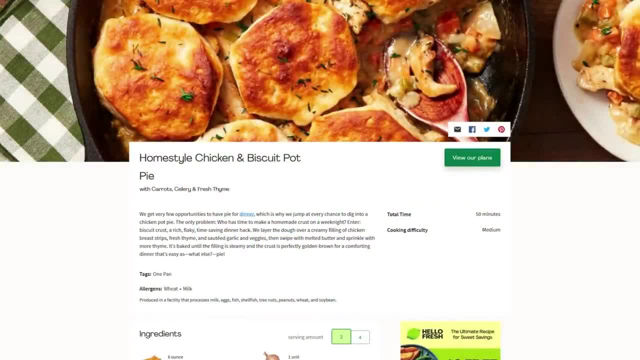 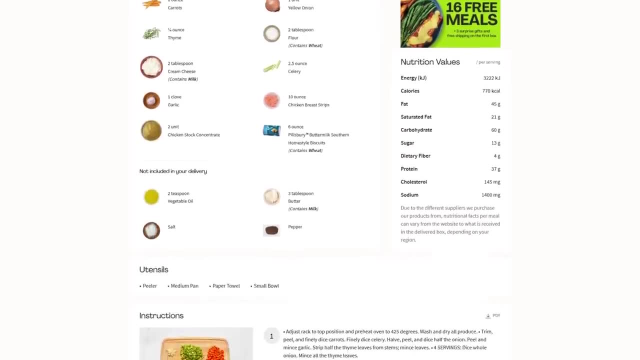 a box arrives on my doorstep with all the ingredients and recipes. For example, this week I made the homestyle chicken and biscuit pot pie, which was pretty quick to make, since all the ingredients came in the exact right quantities, and it was also delicious. 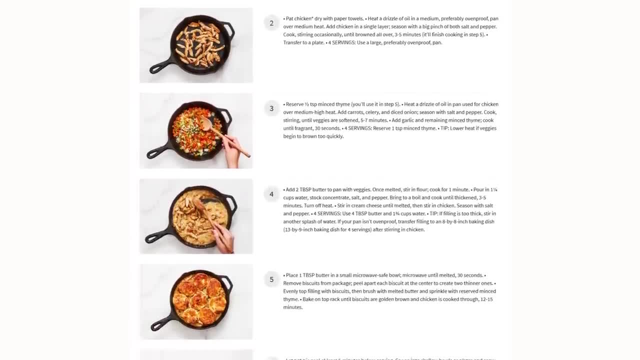 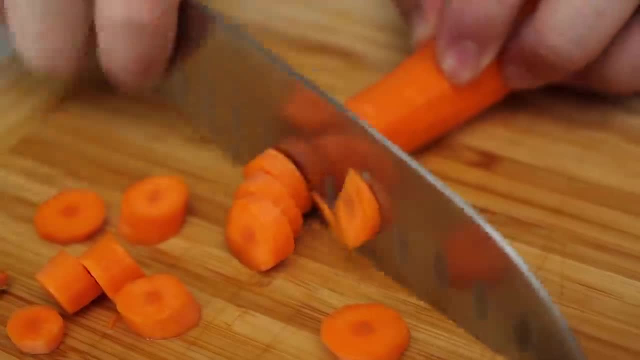 And, to be honest, I've been using HelloFresh for nearly a year now and I have tons of their old recipes here that I've used to prove it. I really do genuinely value the convenience of cutting out shopping, researching recipes and having to do long prep times, while still being able to make. 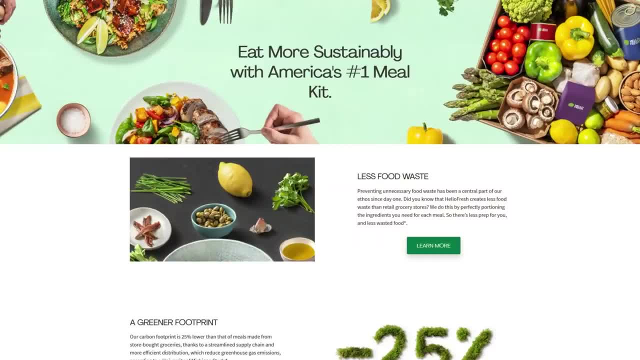 fresh and healthy home-cooked meals. I think it's a great way to start your day. I hope you enjoyed this video and I'll see you in the next one- Bye. To make it even more exciting, though, researchers from the University of Michigan found that 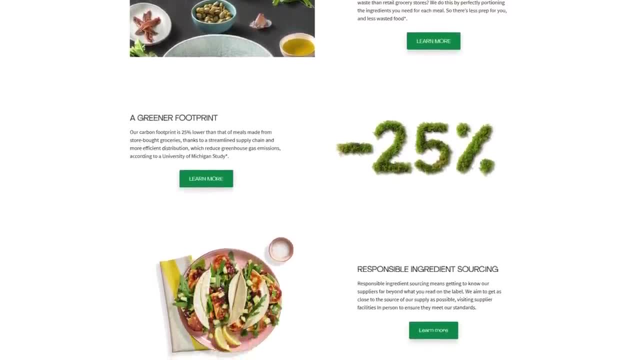 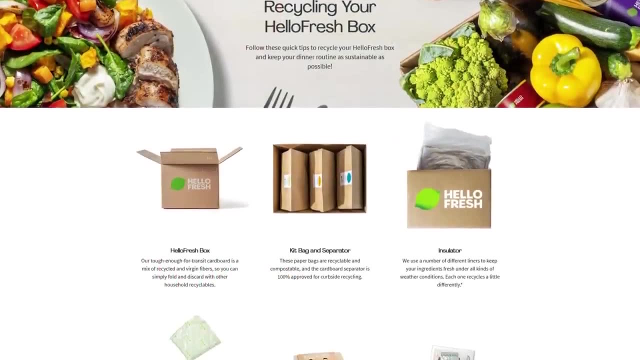 HelloFresh cuts down on food waste by 25% compared with traditional grocery shopping, since you get everything you need in the exact right quantities, and the box it all ships in is made almost entirely out of recyclable or recycled materials. I know that HelloFresh is. 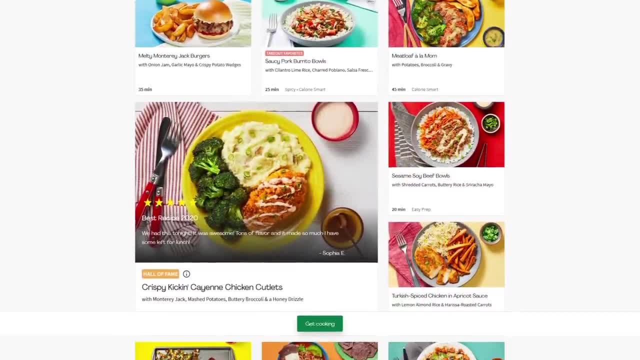 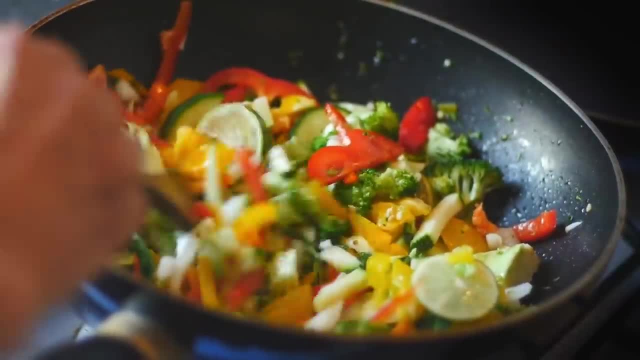 well worth it, since I've been using it for so long. but with this new year, if you're tired of setting unrealistic resolutions for yourself, why not do things differently this time around and regain full control over your own food choices and see if this fits into your lifestyle?